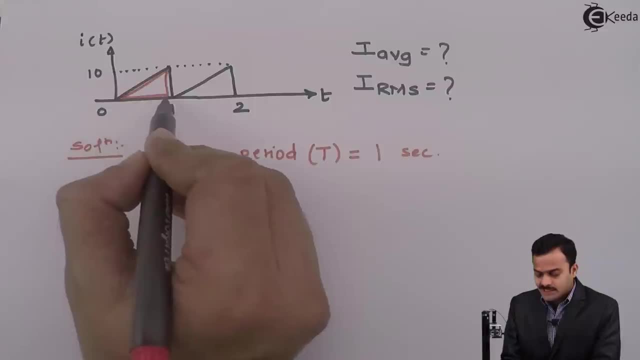 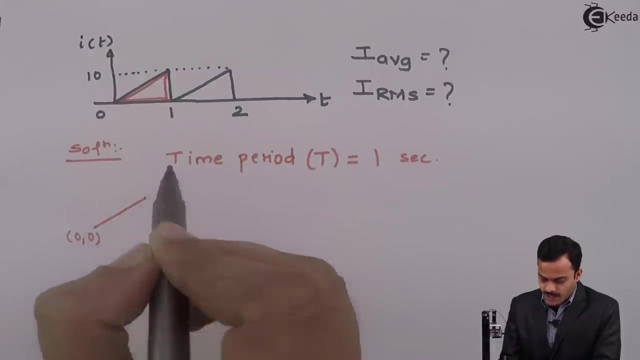 because cycle exists for this much of time. Secondly, we have to write an equation of waveform during a time period, So it is a simple straight line given like this. So coordinates of these two points is 0, 0 and for this point it is 1, 10.. 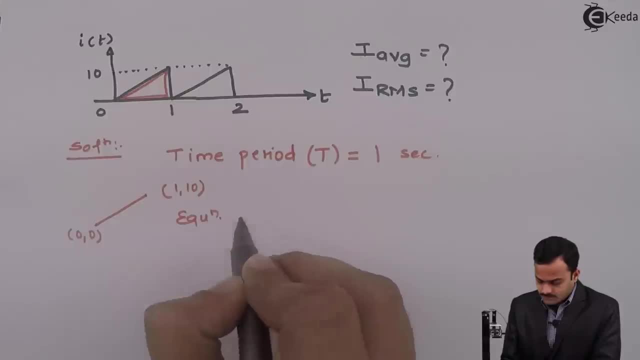 So I can use equation of a straight line. It says: y2 minus y1 upon x2 minus x1, equal to y1 minus y divided by x1 minus x. So here I will consider this as x1, y1.. 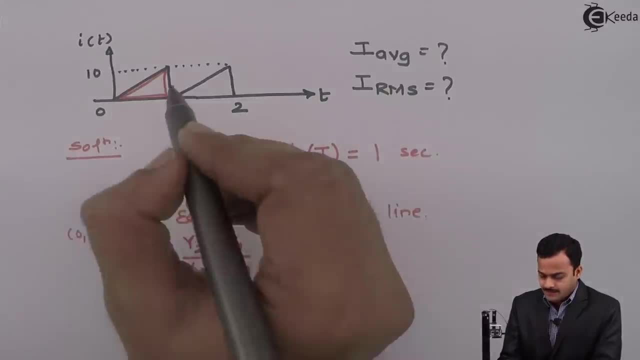 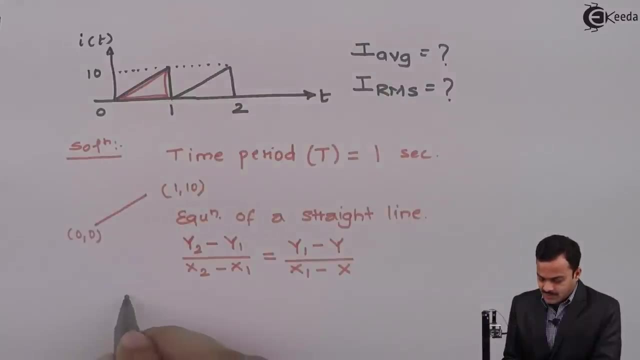 x2, y2, and x axis is T, y axis is I of T. So if I substitute what I will get: y2 is 10, y1 is 0 divided by x2.. x2 is 1, x1 is 0, equal to y1. 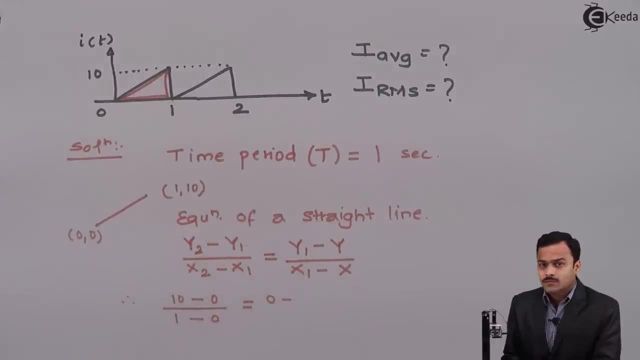 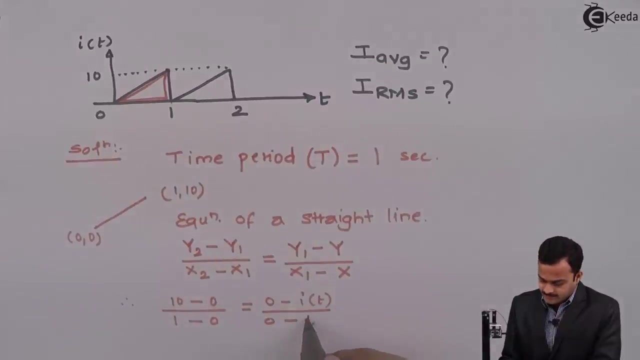 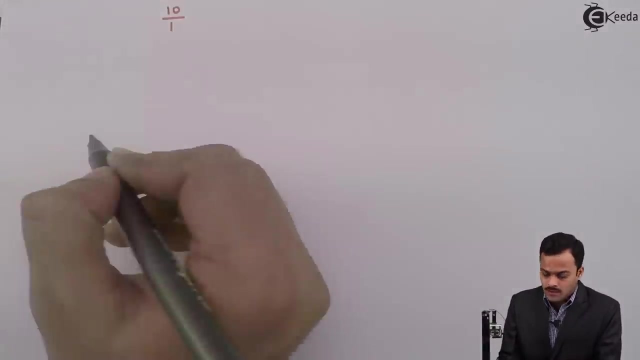 So y1 is 0 again minus y. y is I of T upon x1.. x1 is 0, again minus x. x axis is time axis T. So if I simplify what I will get, 10 upon 1 equal to minus I of T. 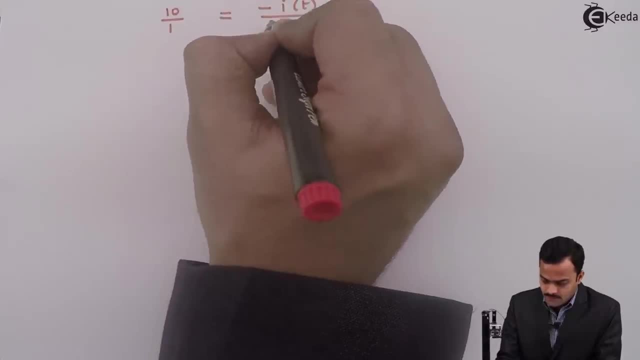 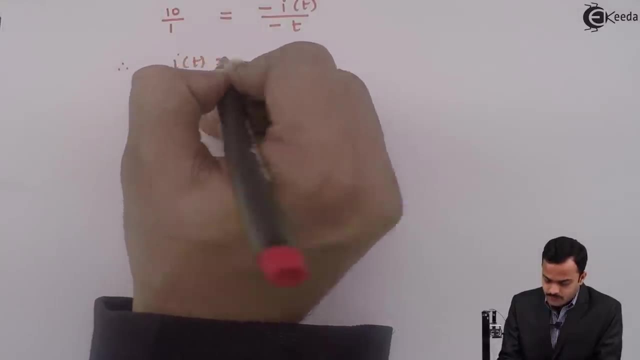 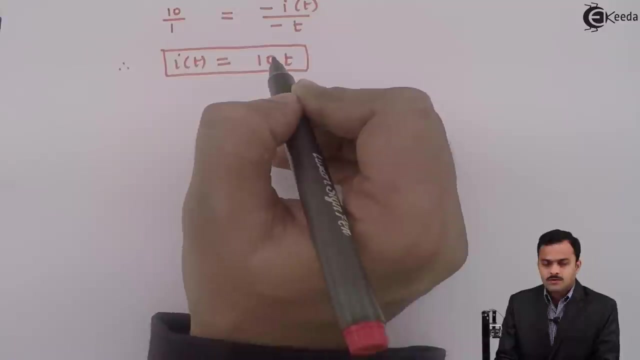 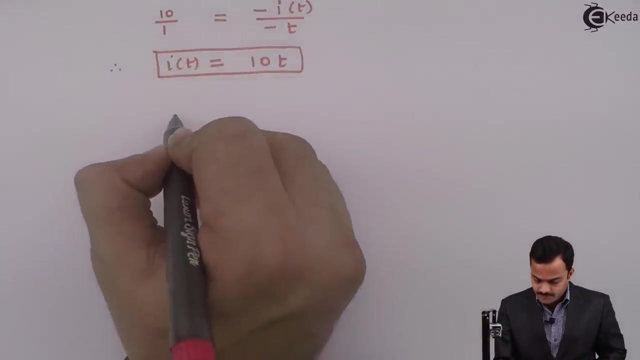 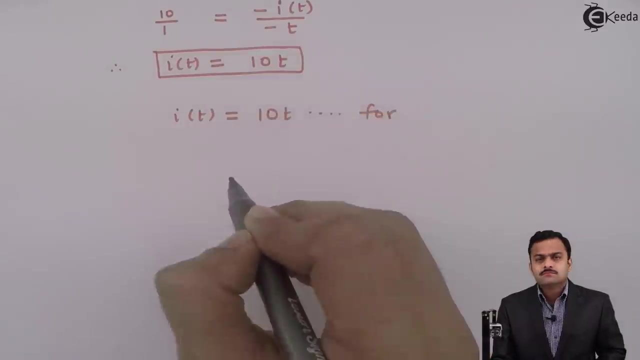 Minus I of T upon minus T. So if I solve, I will get I of T equal to 10 times T. So finally, what I get for this waveform is equation I of T equal to 10 T For T greater than 0 and less than 1.. 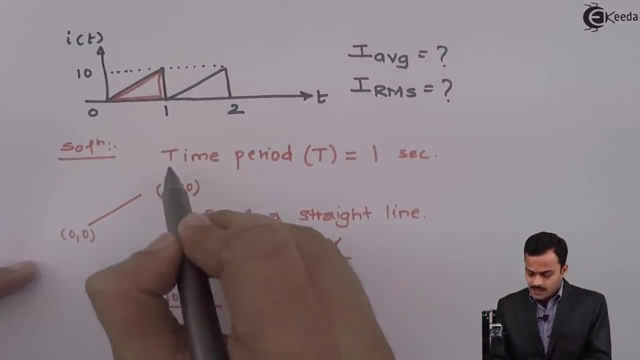 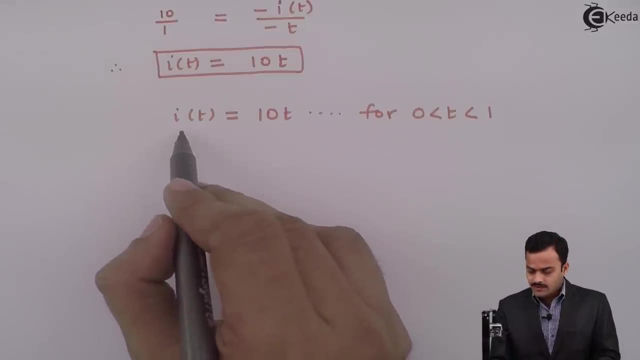 So what I have done? I have decided what is a time period. Secondly, I have got equation of the waveform. Now the problem will become very easy Because we know average value. So average value equal to 1 upon time period. 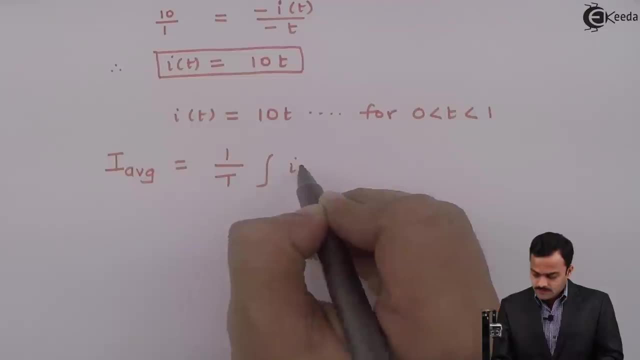 We have to integrate that particular waveform for the time period T. So in this case, what I will get 1 upon 1 and I am having a waveform only from 0 to 1.. So 0 to 1.. 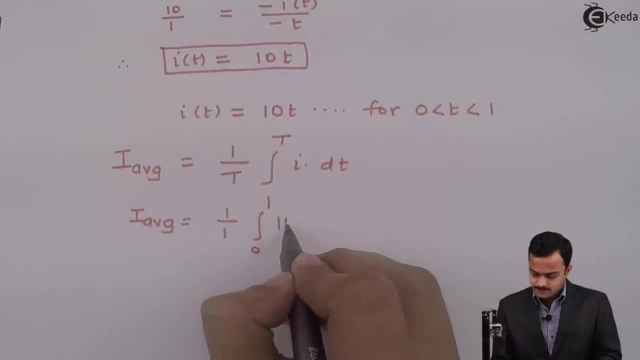 And equation of this I is 10 T, So I average equals 10.. I will take out of a integration. Integration of T is T square by 2.. And let us apply the limits. Lower limit is 0.. Upper limit is 1.. 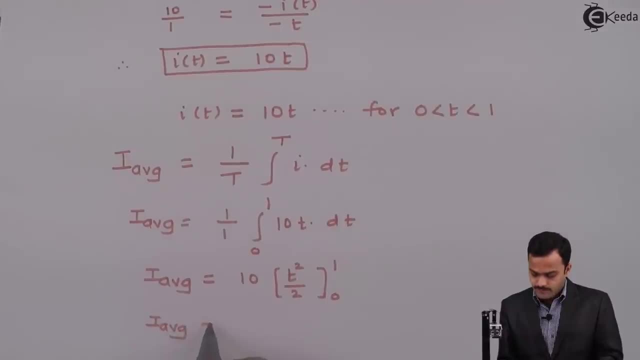 So if I solve, I will get average value as 10 divided by 2 in bracket, 1 square minus 0 square. So ultimately it is 5 only. So it is a 5 ampere. So average value I am getting 5 ampere. 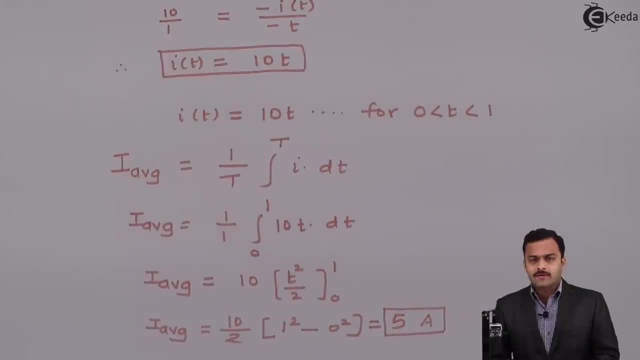 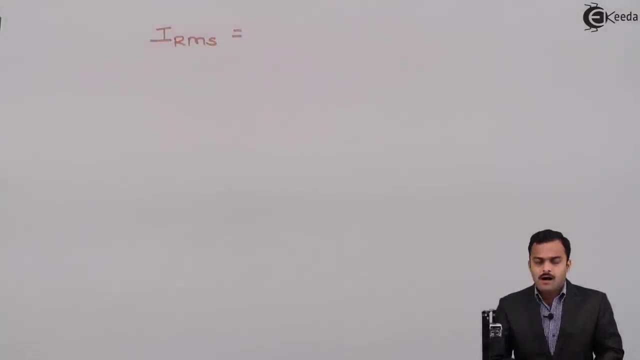 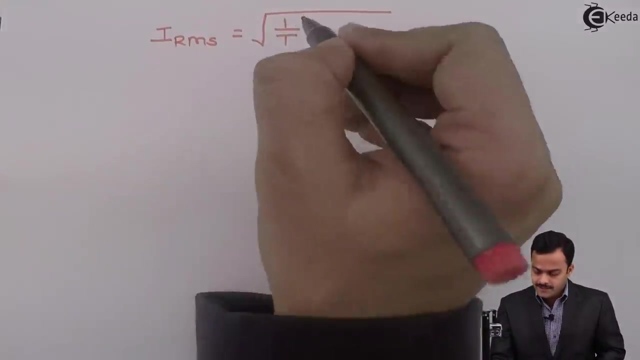 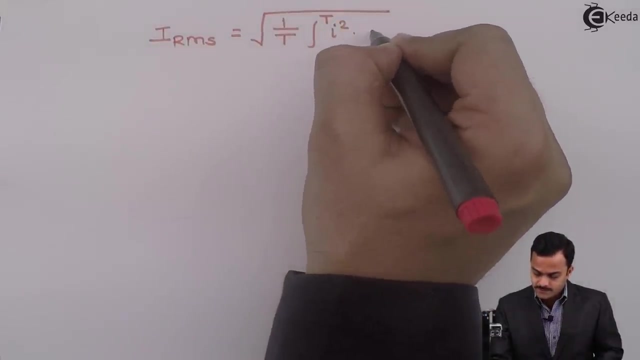 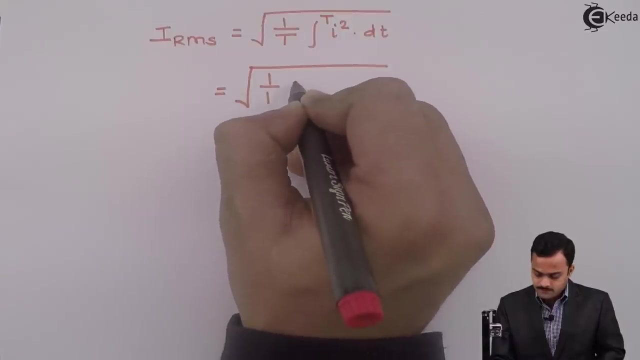 Same way I can get RMS value. So to get RMS value, the formula is: I RMS equals root of 1 by T, integration over a time period T. But this time it is integration of I square. So let us substitute the value 1 upon 1.. 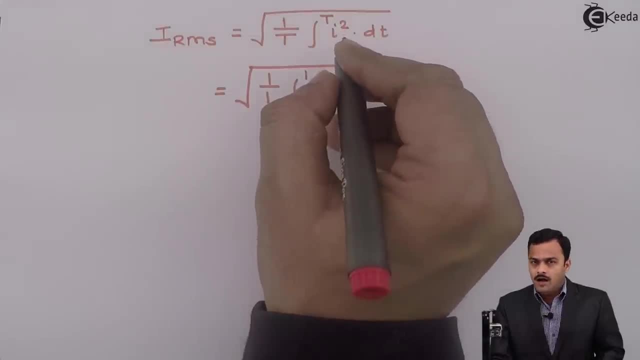 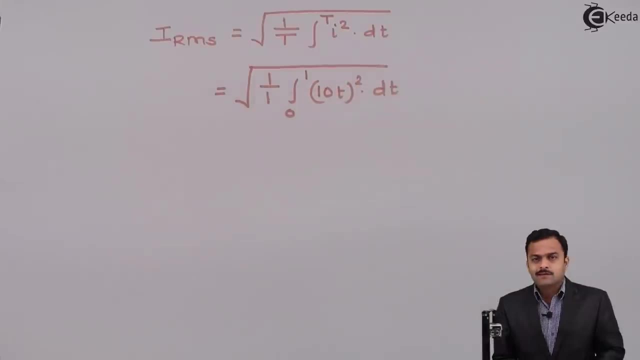 So I am having a waveform only from 0 to 1.. I is 10 T, So 10 T square into DT. So it is root integral 0 to 1, 100 T square. 100 is a constant.